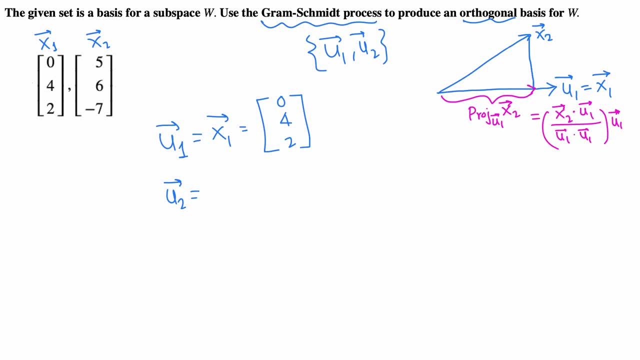 perpendicular to each other. We see u2 has an 평 u1 and so here it's perpendicular to x1. now we want to find a vector perpendicular to x1, so this vector, pretty much, So we find the projection of x2 on to u1, or x1, first vector, that's the projection vector, and it will be always in this direction, this one up to here, given by this formula. then we subtract this projection from this x2.ным. we subtract 2 from this x1. so we Subtract this projection of x2. then we Subtract this projection. now, we subtract 2 from X1 and we Subtract this vector from this X2.. 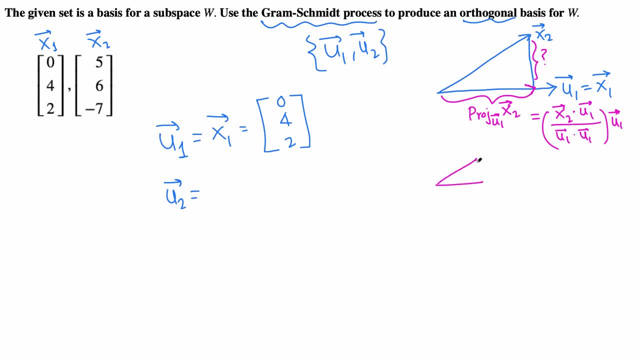 projection from x2. so we have these three vectors pretty much and this is going this way, plus this way is this. but if we subtract this from this, we get this. So this projection, this is scalar number for this question. this one is same as u1. we can calculate: just find the dot product of x2 with u1 multiply we. 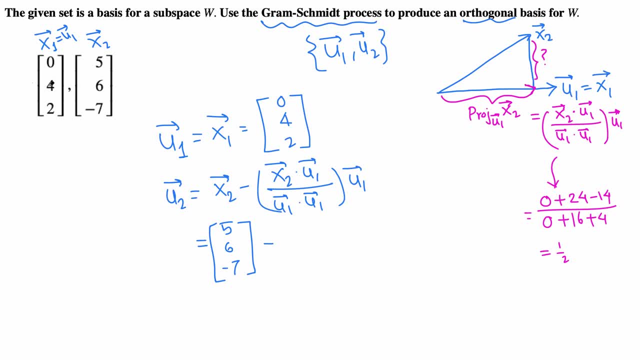 get this: u1, dot u1. multiply u1 with yourself, we get this. so 1 half of u1. so this number is 1 half. u1 is first vector, which is 0, 4, 2.. Now 1 half of 0, 4, 2 means. 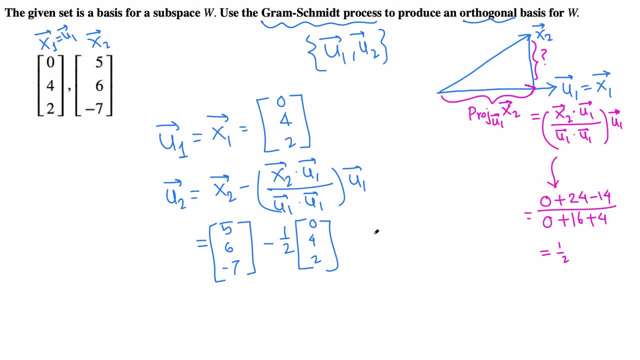 1 half times 0, 1 half times 4, 1 half times 2 and we're gonna get the vector. so 1 half times 0 is just 0, 5 minus 0 is 5, 6 minus 1 half of 4, 1. 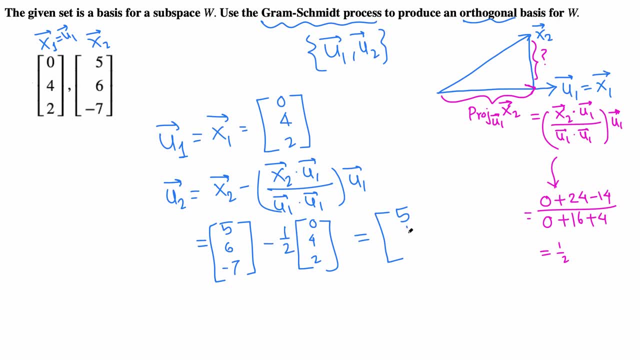 half of 4 is 2, 6 minus 2 is 4, 1 half of 2 is 1, negative 7 minus 1, negative 8.. So u1 and u2 forms an orthogonal basis. You can check. 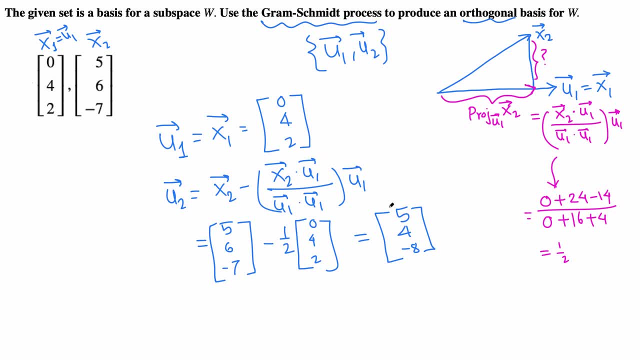 if we, if you, if we multiply these two vectors, u1 and u2, the inner product or dot product is 0.. So u1, u2 is the answer.